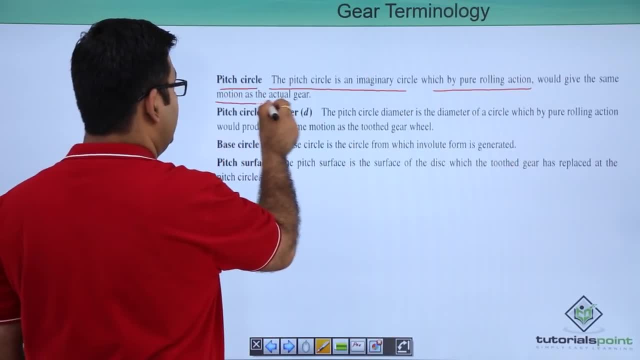 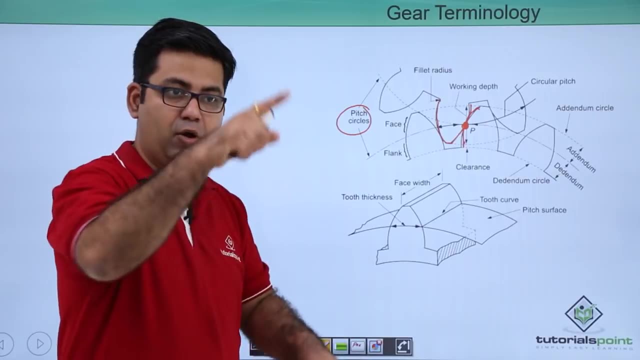 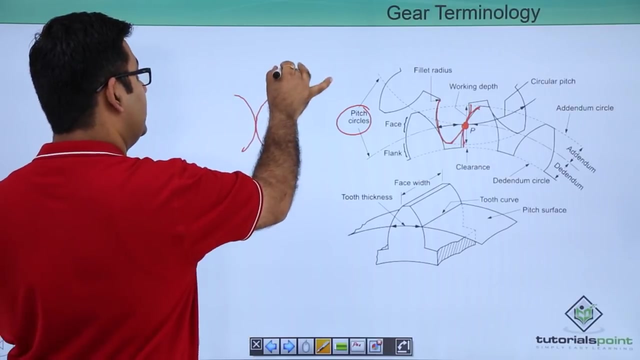 Which by pure rolling action, It would give the same motion as the actual gear. So in some cases we can just get rid of these corrugated projections and we can just draw these two pitch points, the pitch circle. So this is PC1 and this is PC2.. 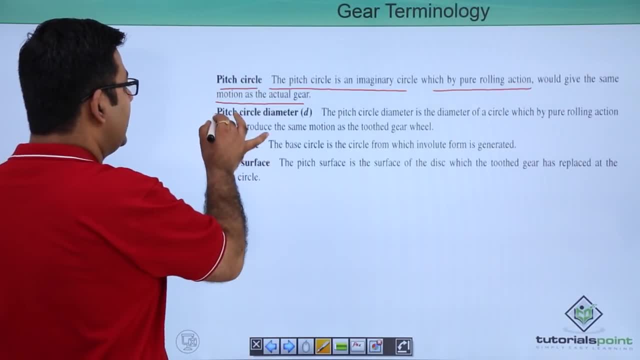 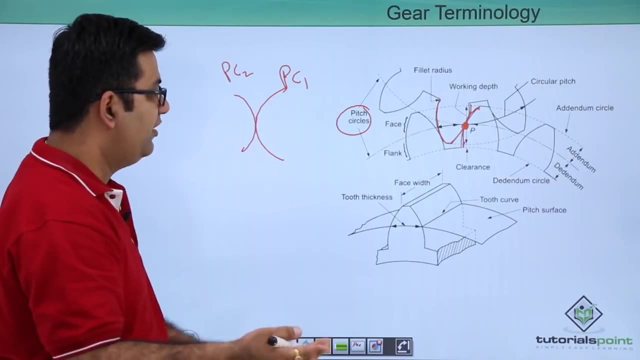 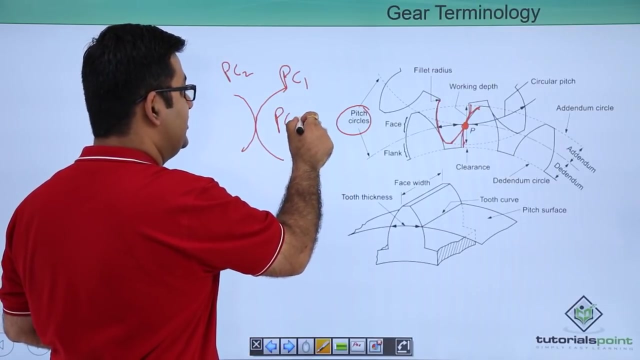 Alright. Next is the pitch circle diameter, or PCD. So the diameter of this pitch circle is called the pitch circle diameter. Very simple as that. So whenever we have to commercially specify the size of a gear, we specify it in terms of PCD or the pitch circle diameter. 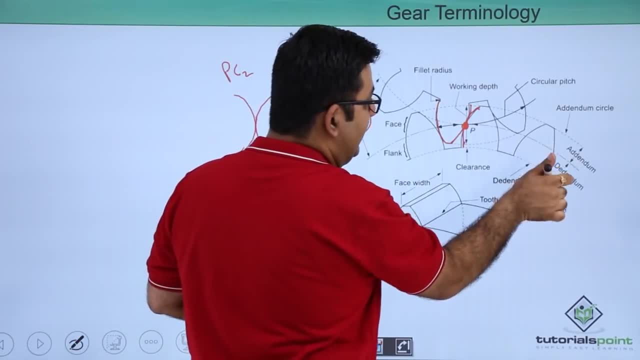 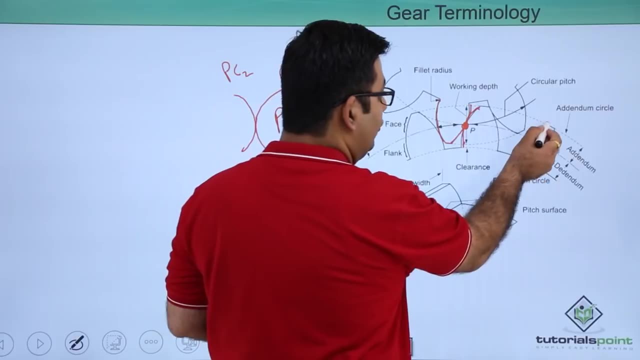 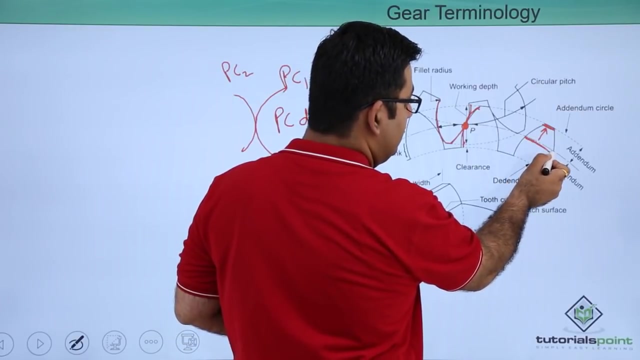 Okay, Now when you go radially above the pitch circle, okay, this radial distance from the pitch circle up to the top of the tooth is called addendum. So this is the pitch circle. You go radially upwards, You go to the top. 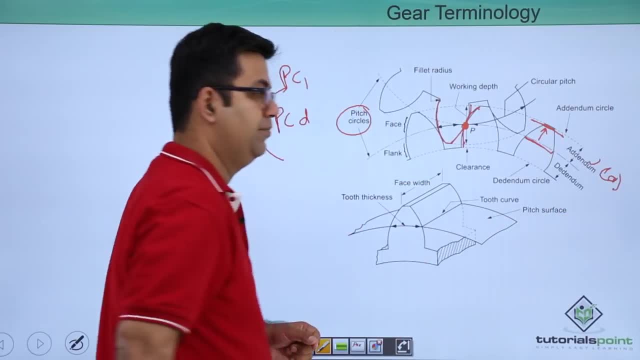 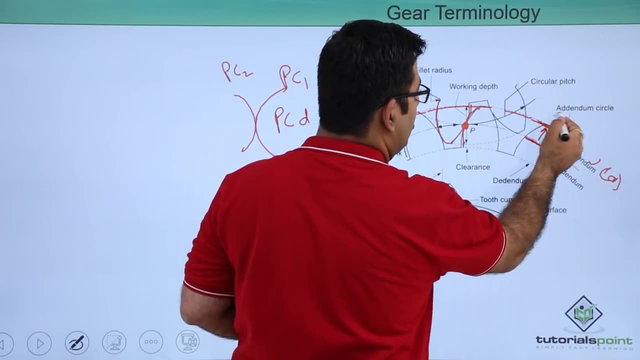 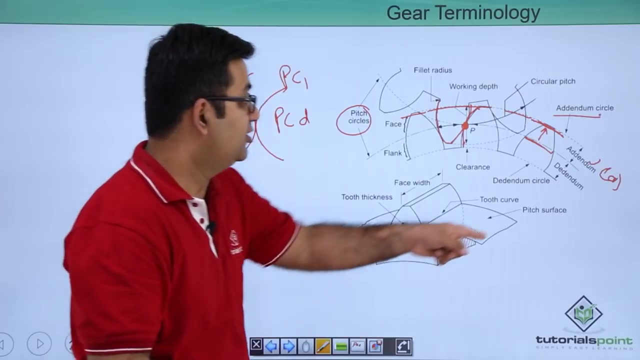 You go to the bottom of the tooth. This distance is the addendum A, And the circle which is joining all the top surfaces of the gear is called the addendum circle. So there is a radial distance between the pitch circle and the addendum circle and that is called addendum. 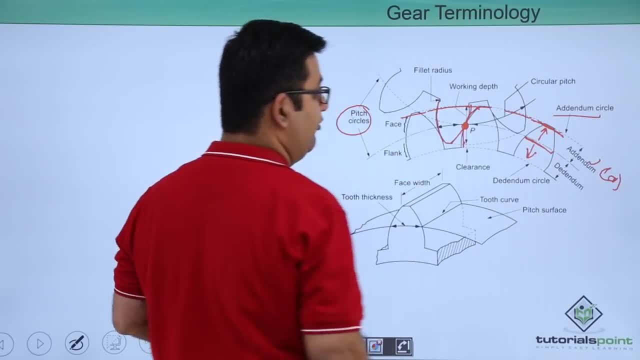 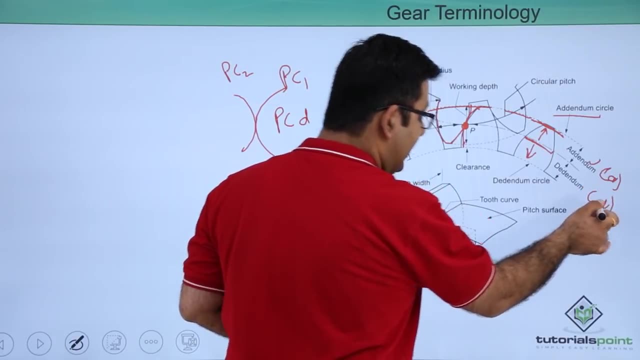 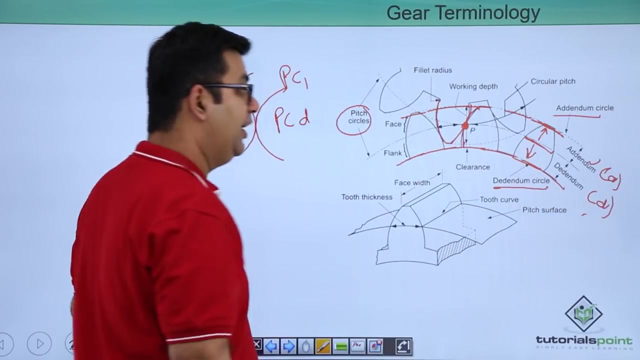 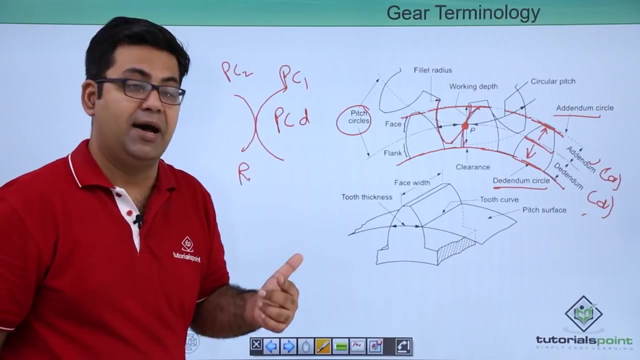 Similarly, if you go radially downwards from the pitch circle, you go down by an amount called Addendum. You come to the bottom of the circle. This bottom circle is called the addendum circle. So let us say, if you have the pitch circle radius as capital R. 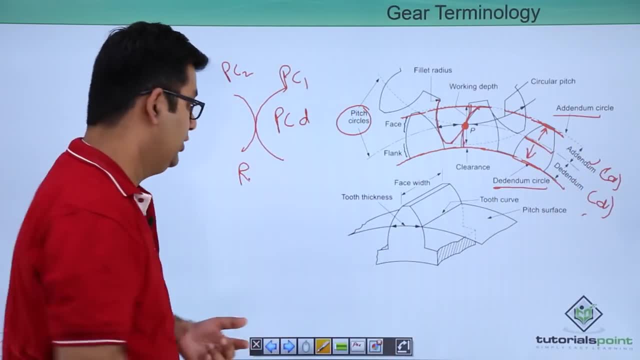 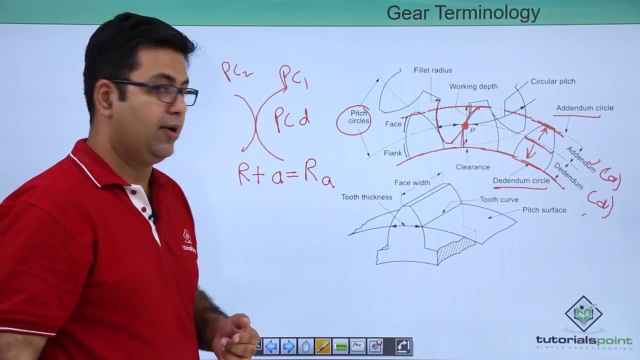 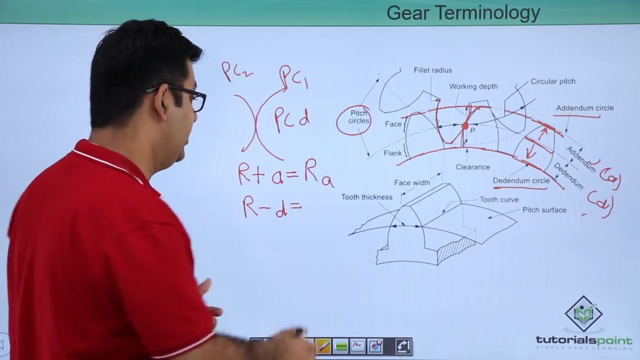 And if I add capital A to it, you get to the addendum circle radius. So if I add A to it, you get RA, Okay, Okay. And if I subtract D from it, D is already your pitch circle diameter. So I just say D dash, you get RD. 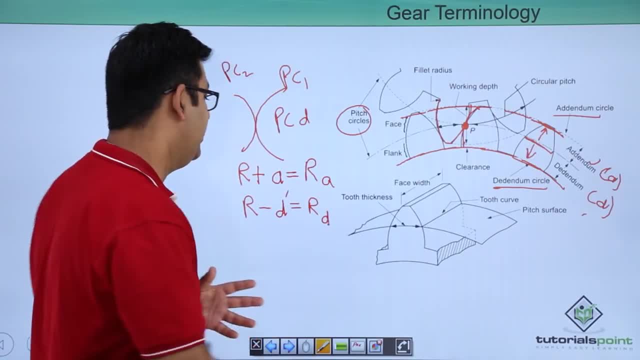 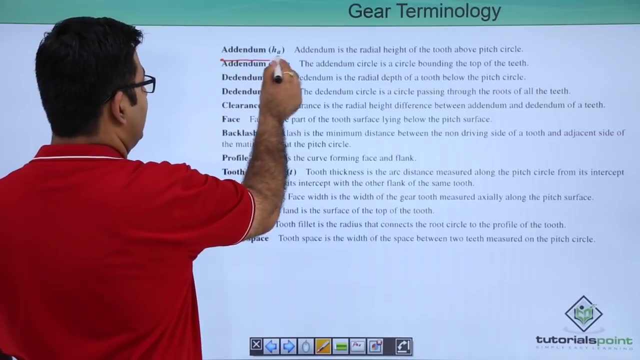 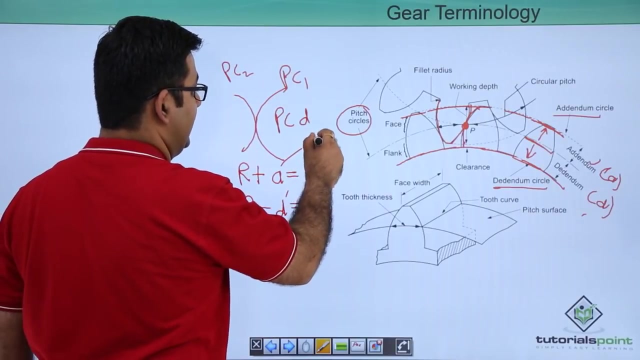 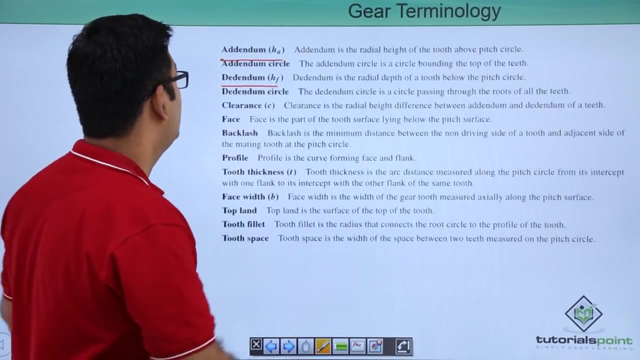 That is the addendum circle radius, where D is the addendum. So if you look at the definition of this, addendum is HA and addendum is HF, So I can write down this as HA and this as HF. So addendum is the radial height, the tooth above the pitch circle. 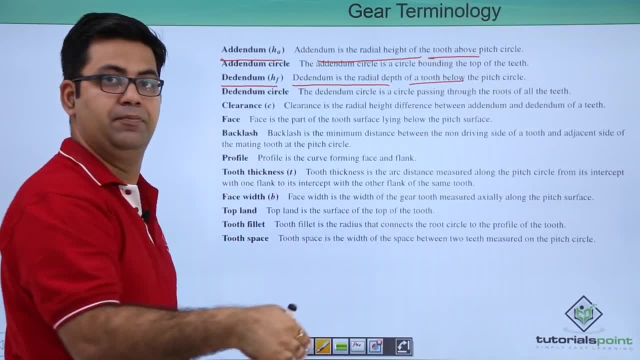 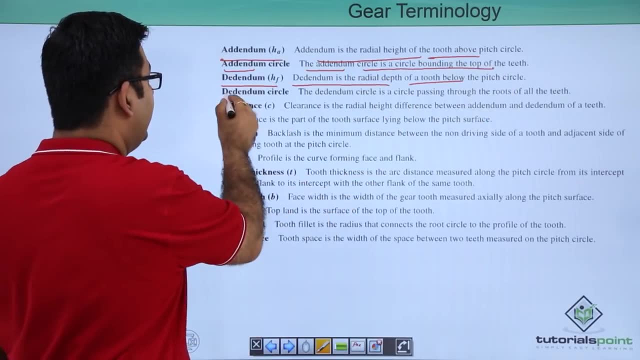 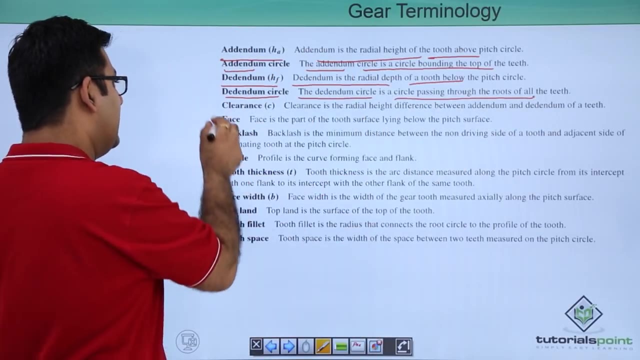 The addendum is the radial depth of a tooth below the pitch circle, And the addendum circle is the circle bounding the top of the teeth, And the addendum circle is the circle passing through the roots of all the teeth. Okay, Then you come to this part: clearance. 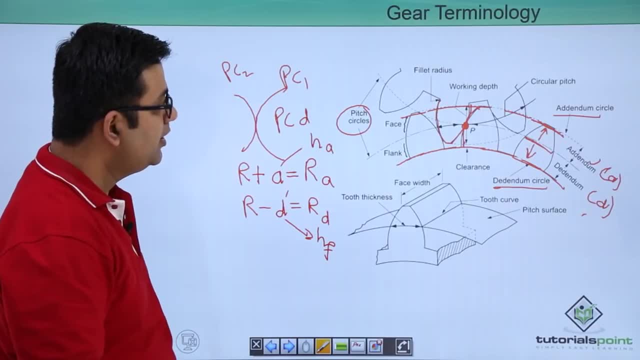 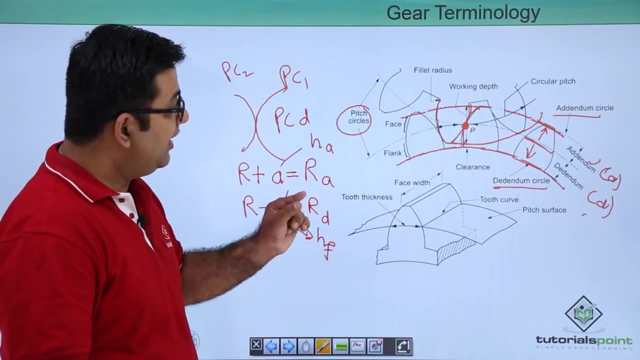 Okay, Let us go to the figure again. You see, You have the addendum circle of the top gear over here And then you have the addendum circle of the bottom gear. These two are not meeting each other. There is a certain amount of gap. 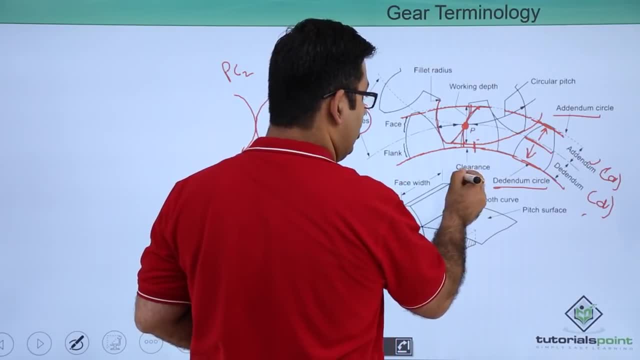 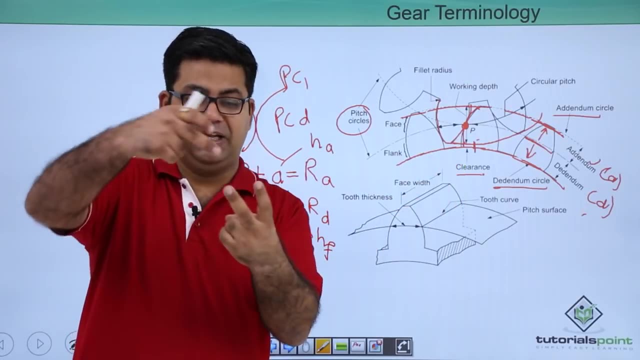 So this gap over here is called the clearance. So if this is the gap between the two teeth on the bottom gear, the top teeth will come like this. So this is how it meets. There is a certain amount of gap in the fingers. 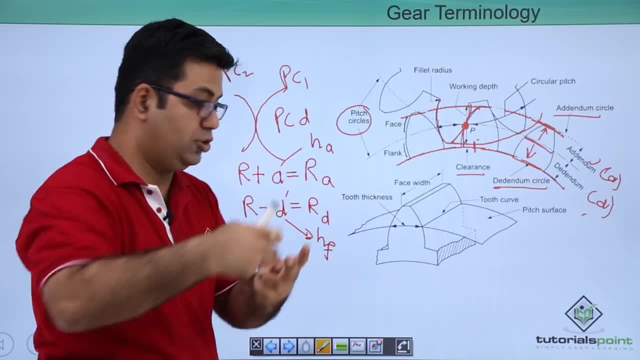 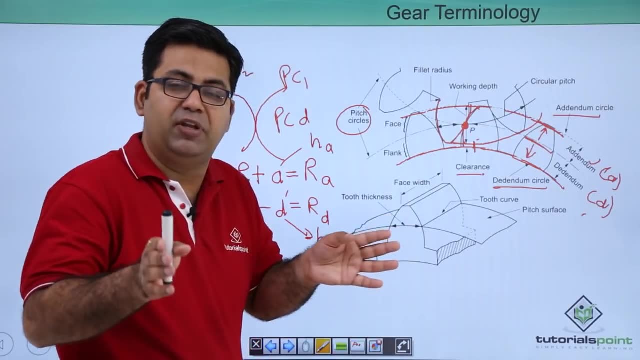 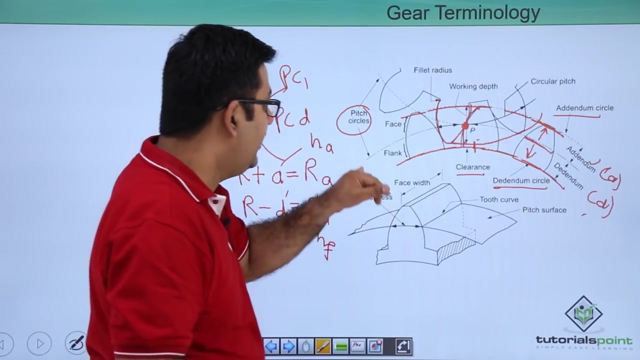 You can see at the bottom. Okay, This is called the clearance. There is no digging. Okay, So that interference has to be avoided. Okay, So as to the strength of the teeth is not reduced. So this is called clearance. That is the radial distance in between the addendum circle and the addendum circle of the two teeth. 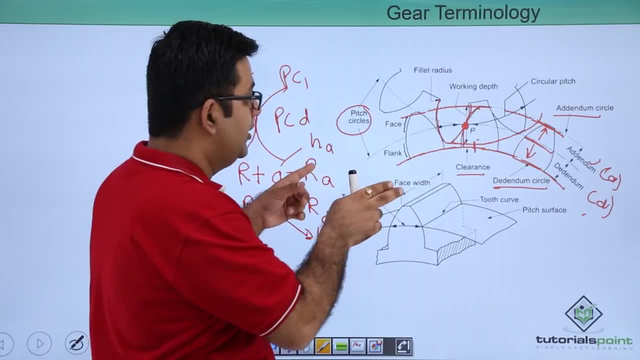 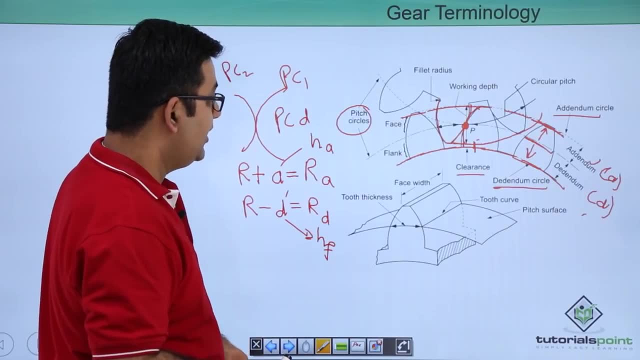 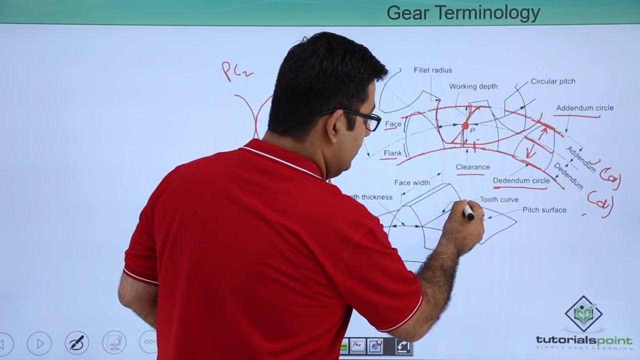 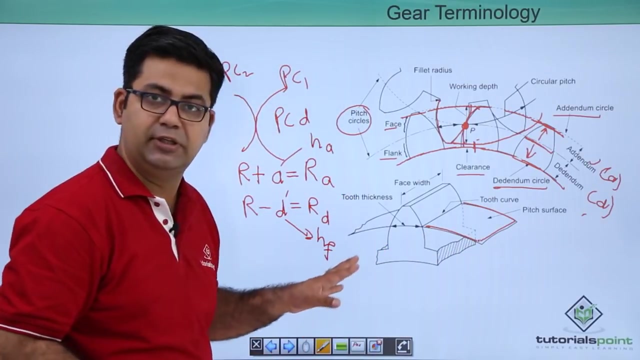 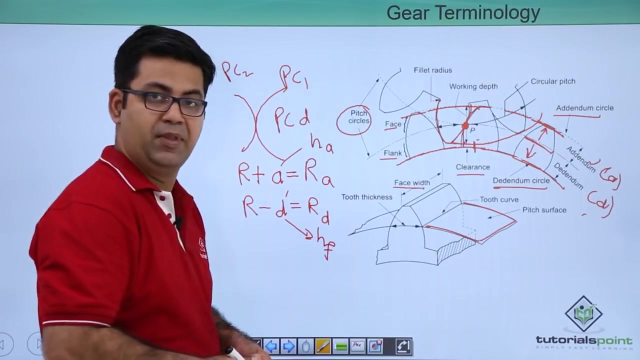 Of the two different gears which are in, you can say which are meeting with each other. Alright, So this is clearance. Then we talk about face and flank. Now, if you look at this surface, this is the pitch surface which is there. if you, if you just take away this teeth, or you take away this tooth and you replace it with the help of a disc of the same face width, your face width is this: 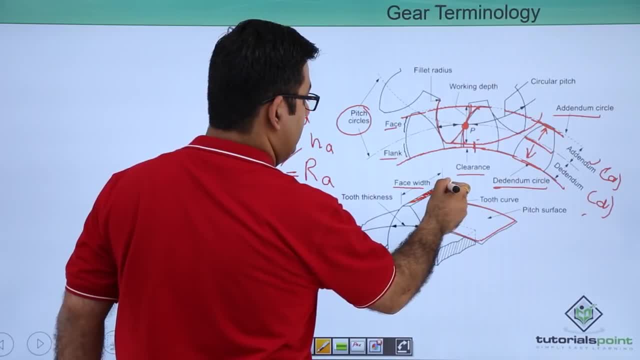 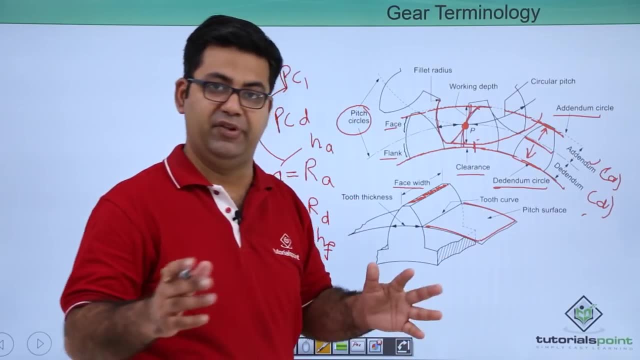 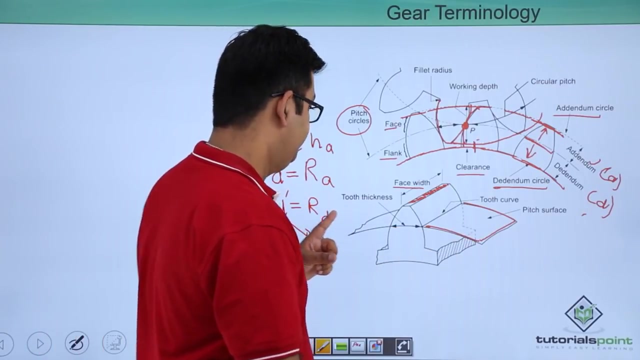 This is the face width. Okay, That surface is the surface, or the top surface of that disc is called the pitch surface because it is passing through all the pitch points. Okay, Now, the part of the tooth above the pitch surface, or the pitch circle, is called the face. 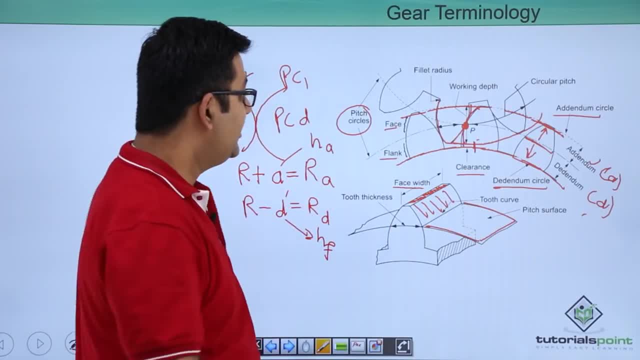 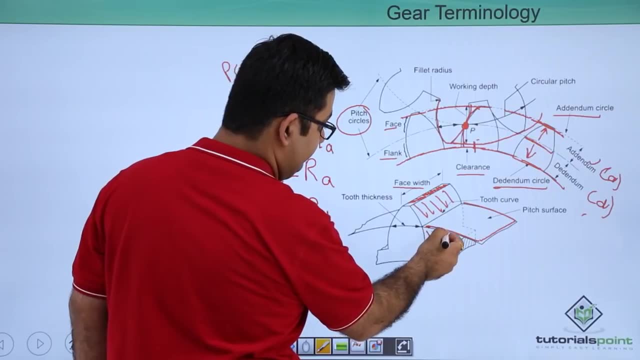 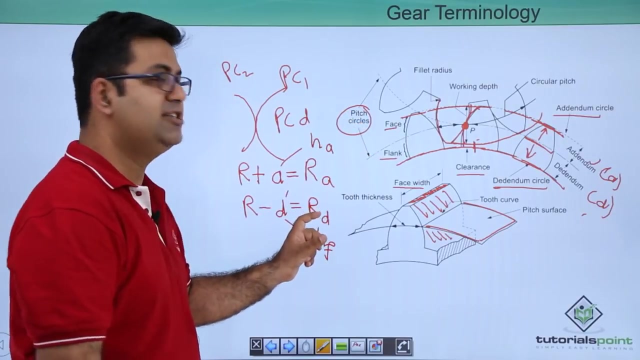 So this part is called the face And the bottom part of the tooth below the pitch circle or the pitch surface. is this, Okay, This one, This one. It is called the flank. Okay, So face is above the pitch circle, Flank is below the pitch circle. 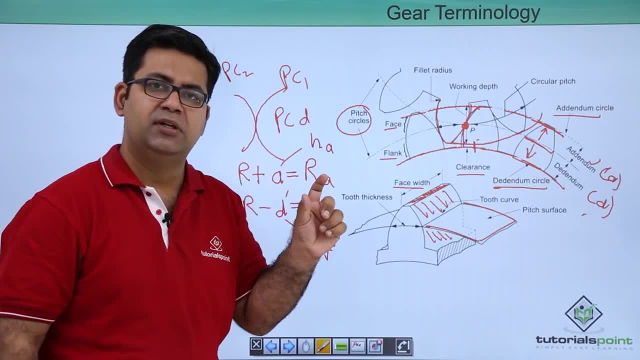 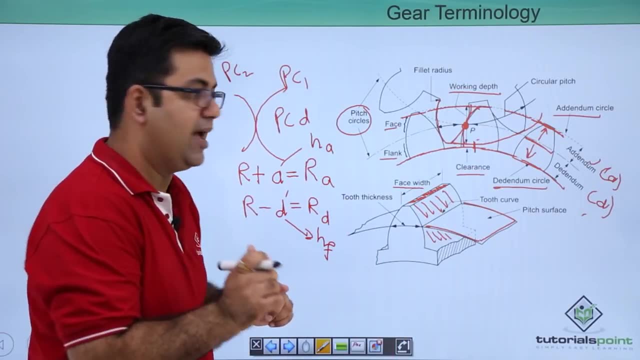 Okay, Then if you talk about the working depth, that is, this particular part, as I told you, there is a certain amount of gap in between the addendum and the addendum circle, So there is a certain amount of gap over here also. 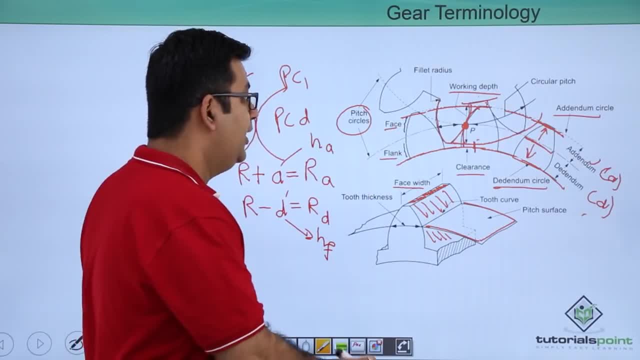 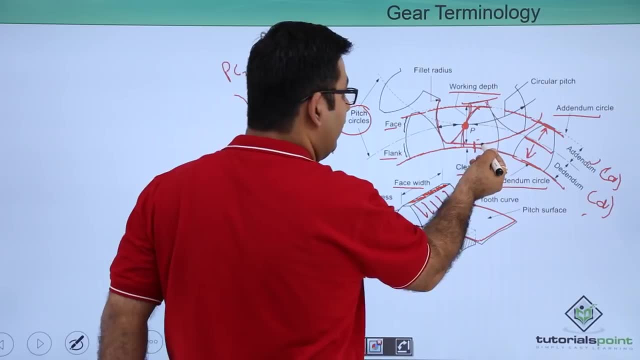 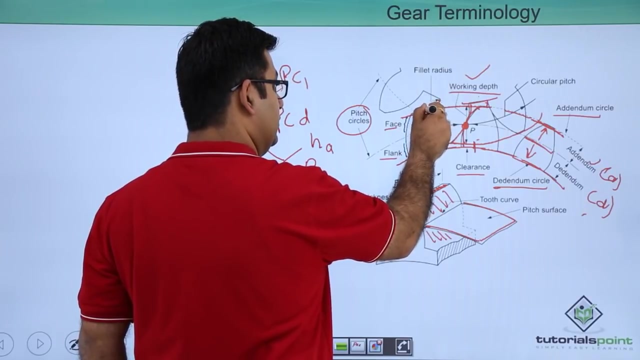 So you have clearance at the bottom and the top gear. Okay, So the distance between the addendum circle of the bottom gear and the addendum circle of the top gear, this is called the working depth. You can see from this point, that is, on the addendum circle. 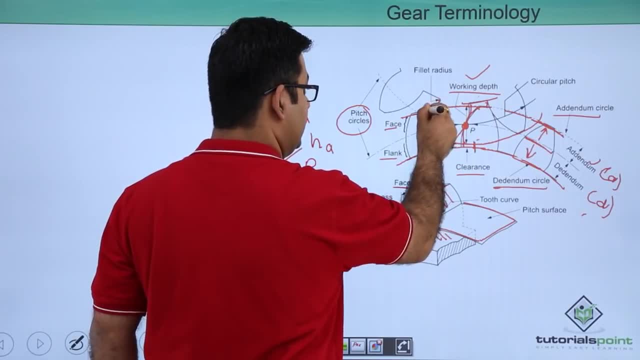 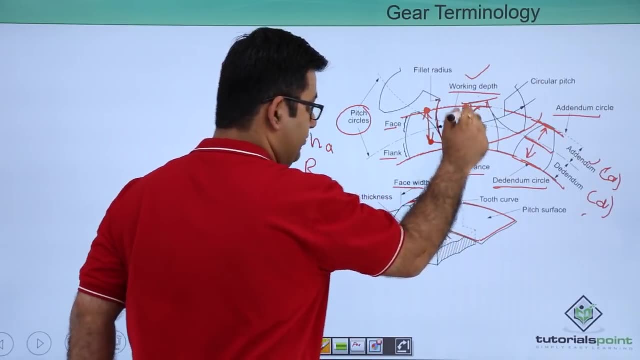 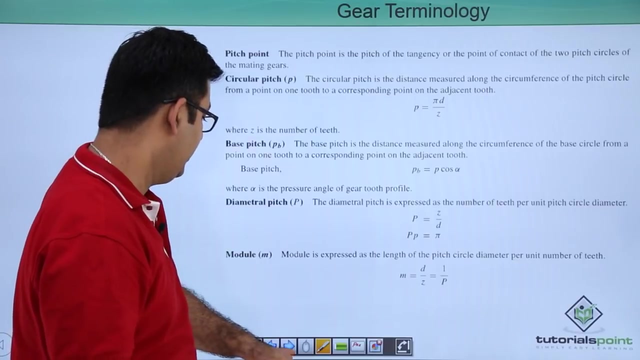 Okay, To this point. This is the working depth Where they are meeting each other. from this point onwards to this point. Okay, That is the working depth. So if you look at the distance working depth, where it is, we have working depth. 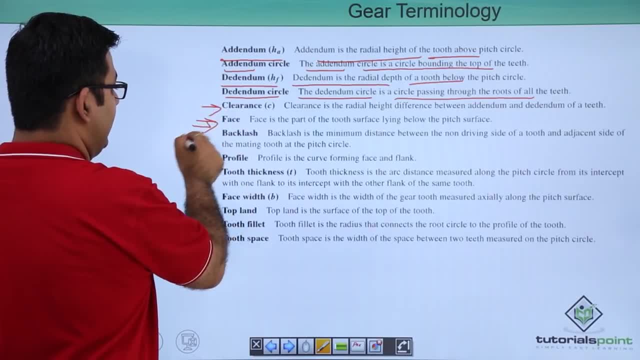 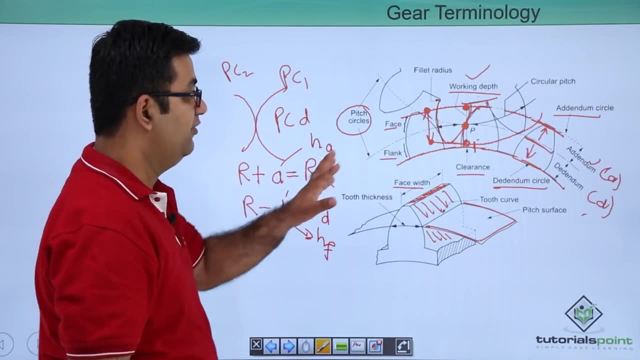 No, we do not have working depth, But we just write down. we have done face, Okay, And we have done the flank as well. Now let us go back to the figure itself. Now, if you look at the distance in between these two points, 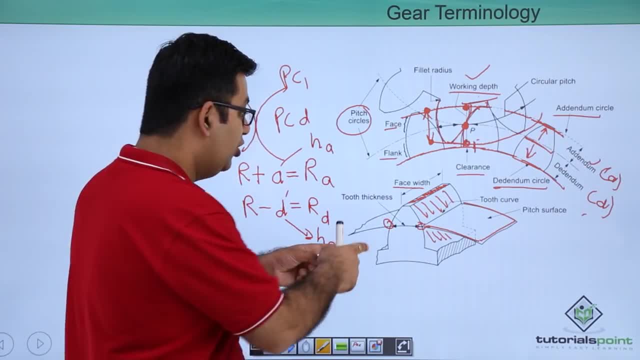 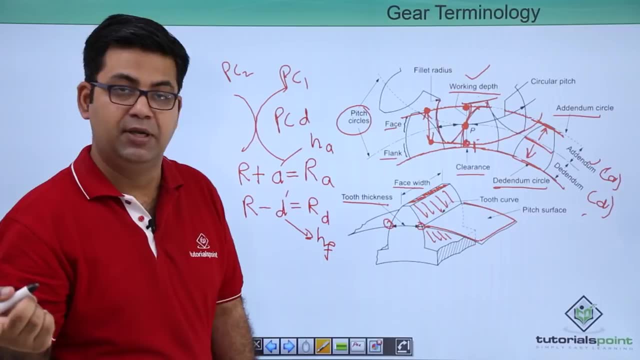 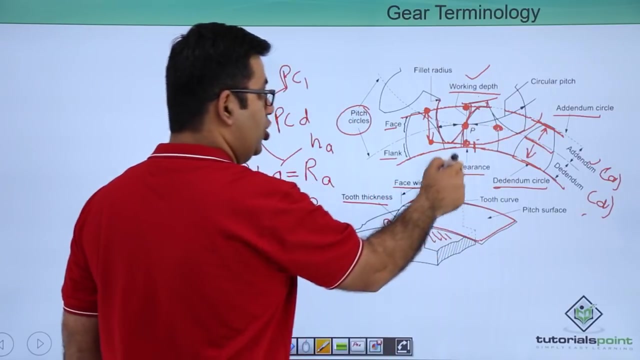 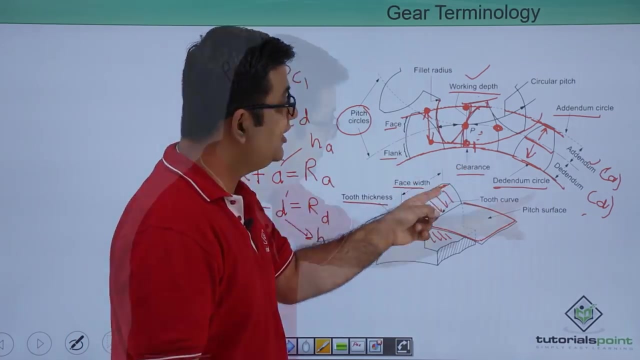 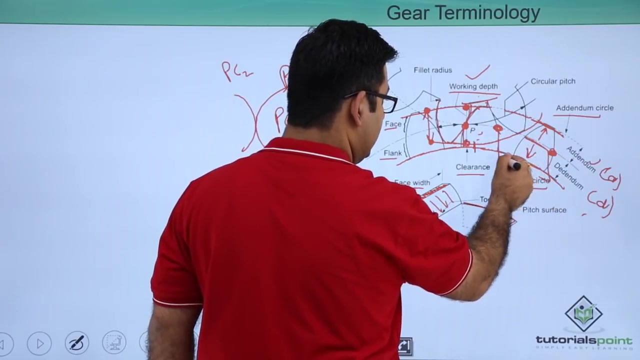 So these two points are on the same tooth, But on the opposite, On the opposite faces, is called the tooth thickness. Alright, Now what is pitch? If you look at this diagram again, if I take this point on this particular tooth and I go to the next tooth and I take the same point on the similar side, that is, this side only if I take this point, this distance is called the pitch. 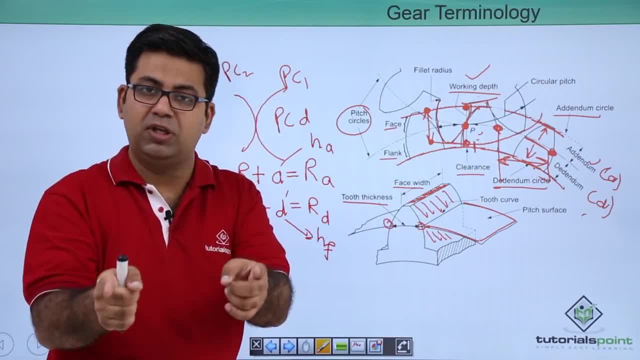 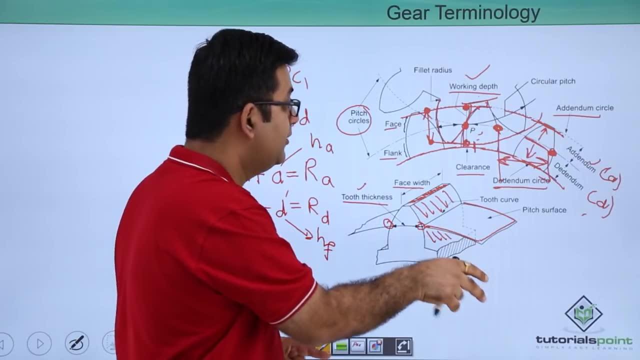 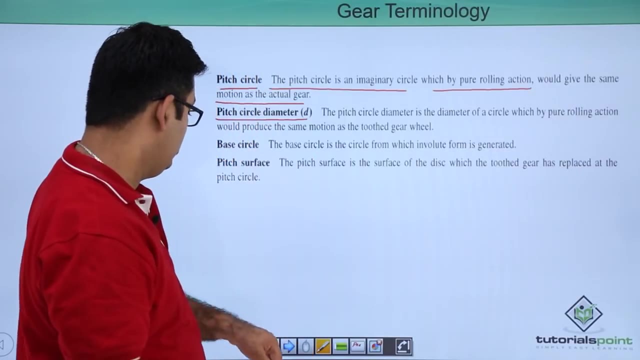 So if you take the same tooth, two points distance is tooth thickness. if you take two different adjacent teeth and the same corresponding point, the distance is called the pitch. Okay, So we have this definition. Pitch point is already taken care of. 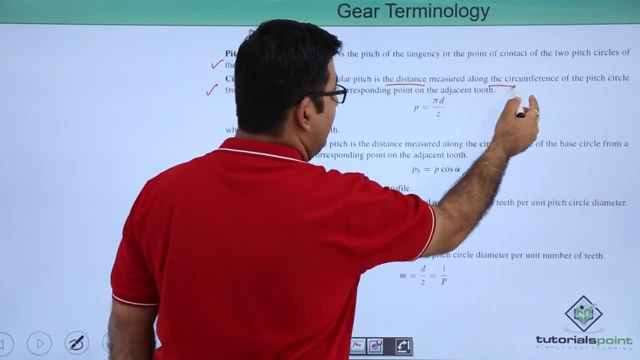 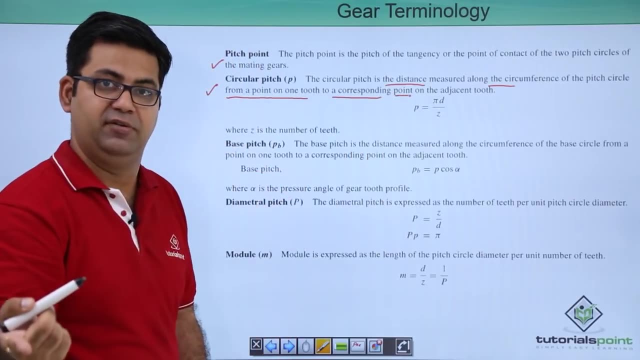 Okay, Circular pitch: the distance measured along the circumference of the pitch circle from a point on one tooth to the other. Okay, To corresponding point on the adjacent tooth. We have just done this, So if you have to draw it. so this is the first tooth. 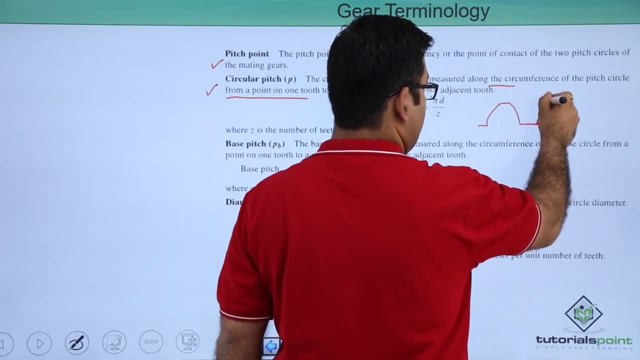 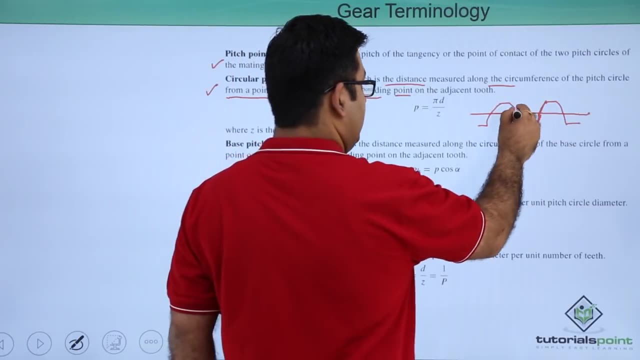 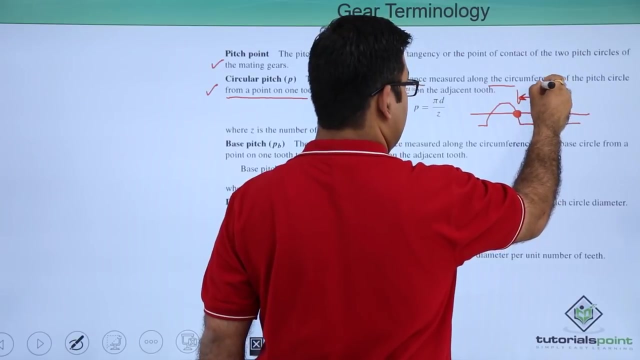 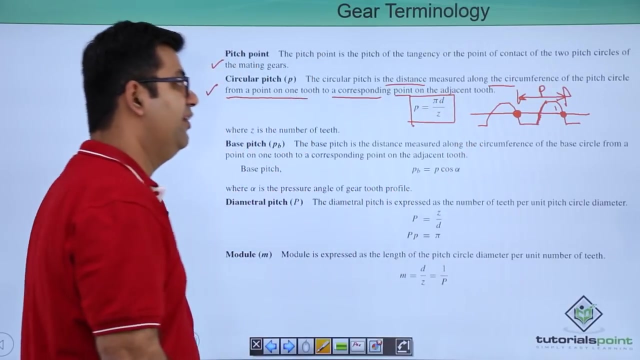 The adjacent would be like this: Okay, So if I take a point over here, this is the pitch circle line. So this point and this point corresponding points. this distance is called the circular pitch And the mathematical formula is pi d upon z, where d is the pcd and z is the number of teeth in that particular gear. 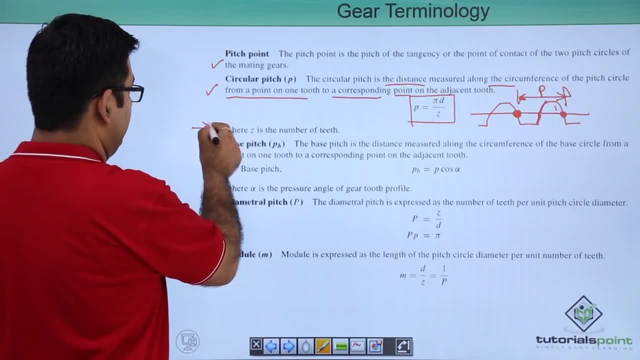 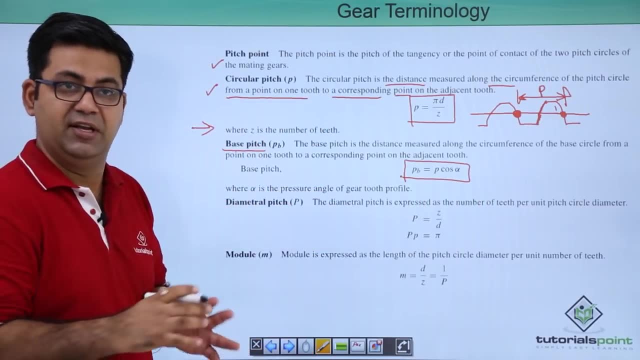 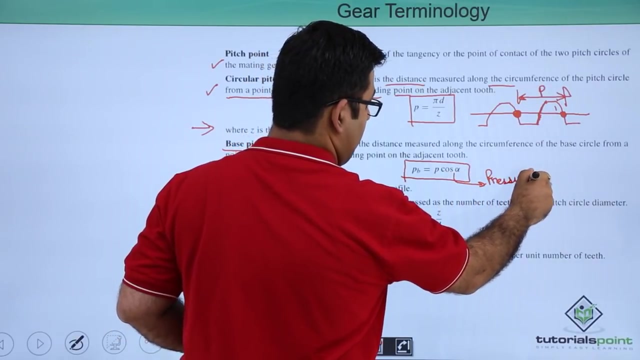 Okay, Make a note of this. And then you have the base pitch. Base pitch is measured with the formula, which is: pb is equal to p cos alpha. Remember this. Alpha over here is the pressure angle. Okay, We will talk about pressure angle in a different video. 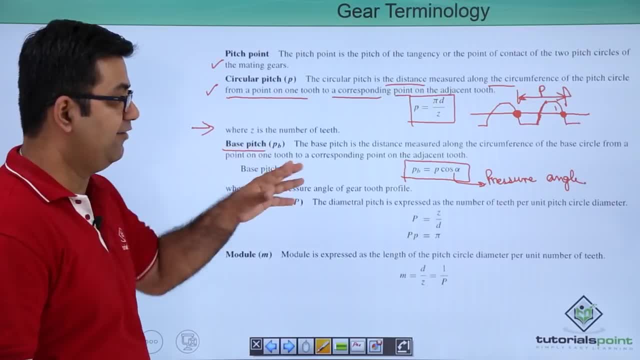 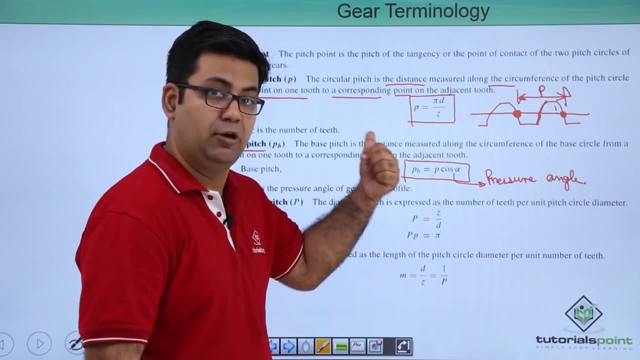 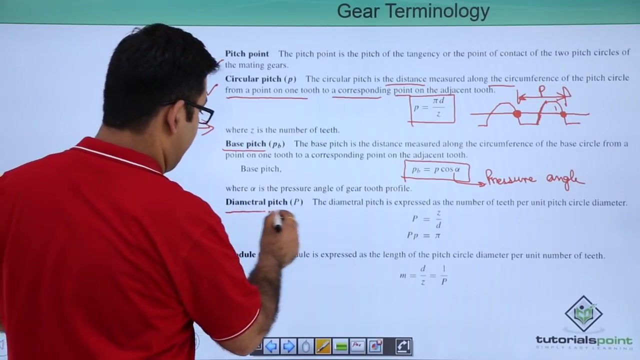 Not over here, But remember this: that base pitch is p, cos alpha, where p is the pitch. Throttler pitch, as discussed in the point above, And pressure angle: we will discuss in some other video. Okay, Then we have the diametral pitch. 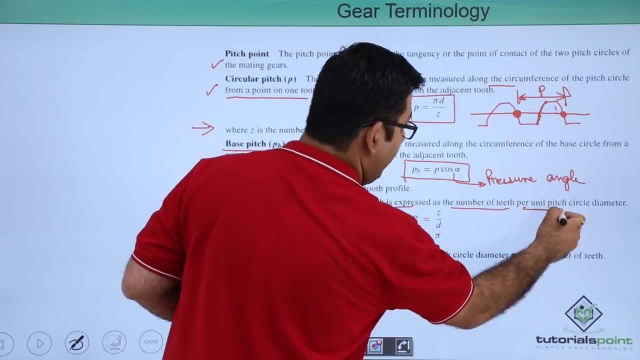 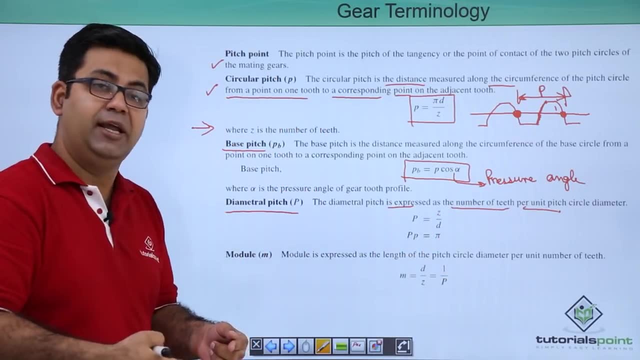 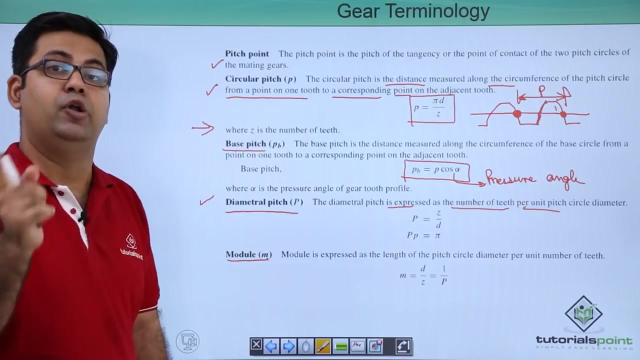 Diametral pitch is expressed as the number of teeth per unit pitch circle diameter. So you take the number of teeth Divided by the pcd, you get your diametral pitch. Now a very important point you have, that is, module. 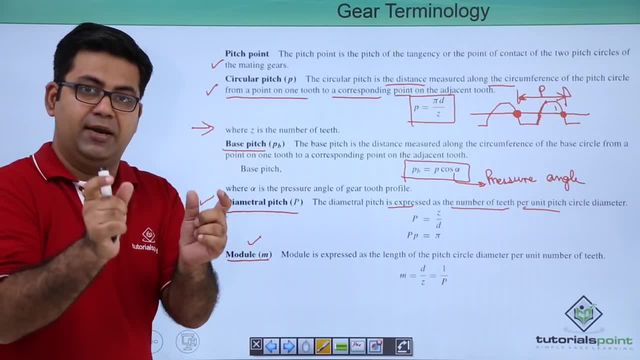 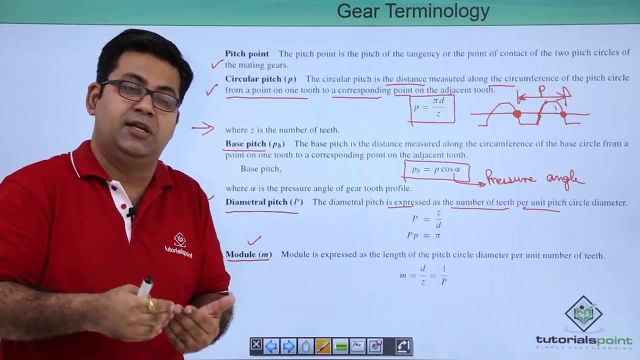 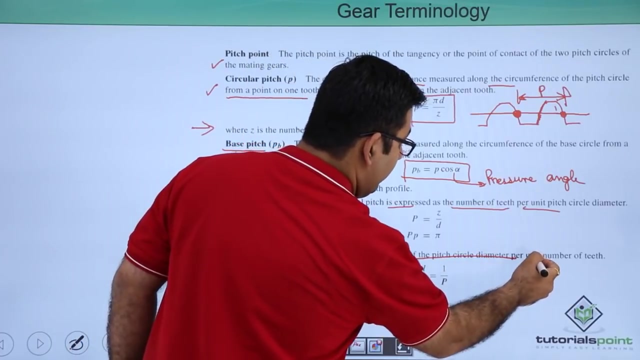 Now, module is a geometrical, we can say- figure which is used to basically design gears. So two mating gears should have the same module. So module is expressed as the length of the pitch circle diameter per unit number of teeth. So basically it is the opposite of the diametral pitch. 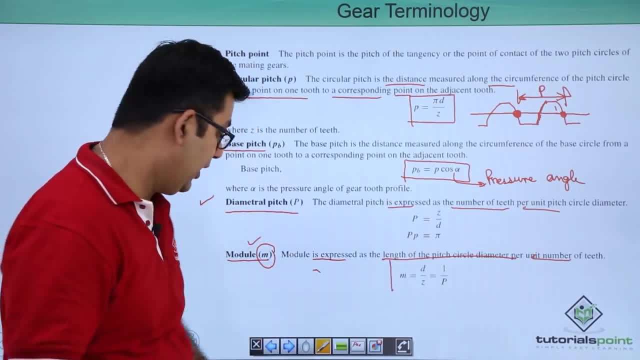 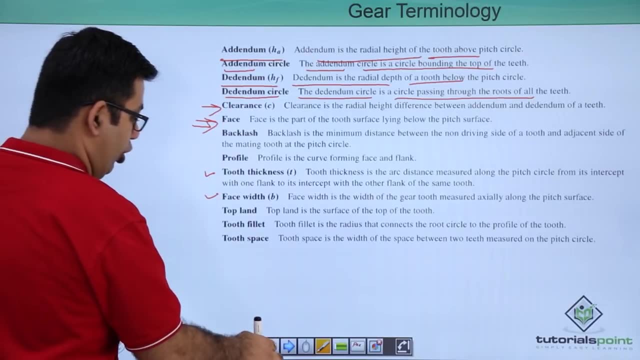 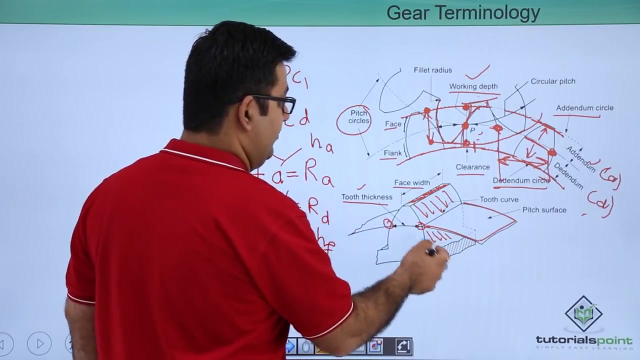 So it is d by z. Okay, Make a note of this. Then we have talked about tooth thickness. We have talked about the face width, Top land. if you go back Top land, Your top land is basically this. only This particular surface is called the top land. 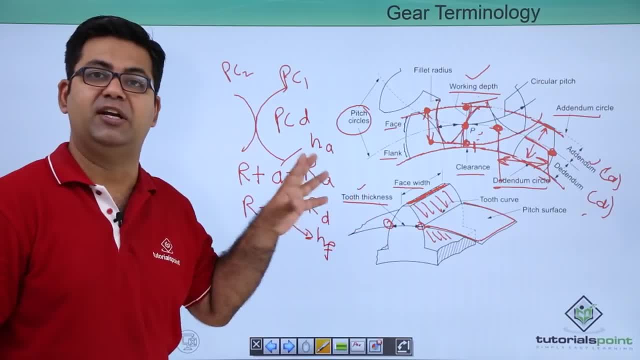 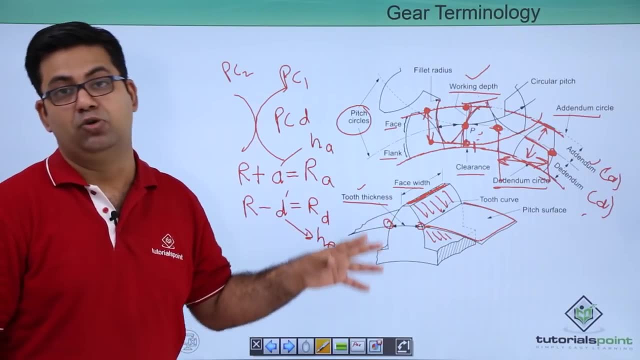 Okay, So these are some very important points for you to understand and remember In the topic of gears and which will be used throughout the analysis on gears. So I hope you have understood this. Now. let's move on to the next video and talk about the law of gearing.